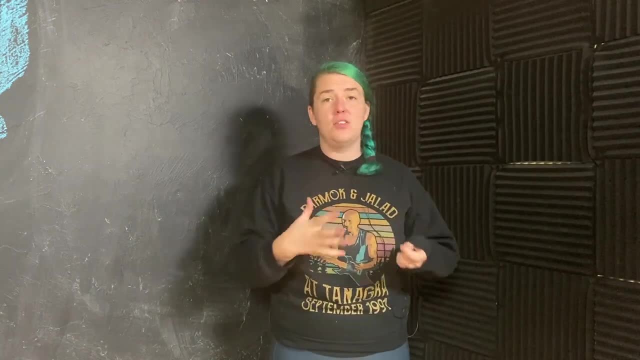 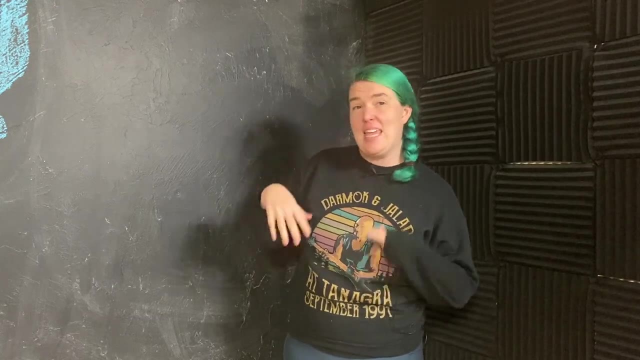 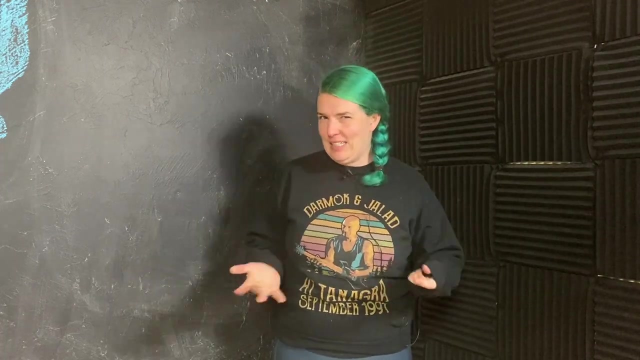 dig into this topic, but if we're going to get anything other than surface level, we've got to do some math. I will explain the math as simply as I can whenever we get to it, so that you'll at least understand what I'm doing, if maybe not exactly how I did it. 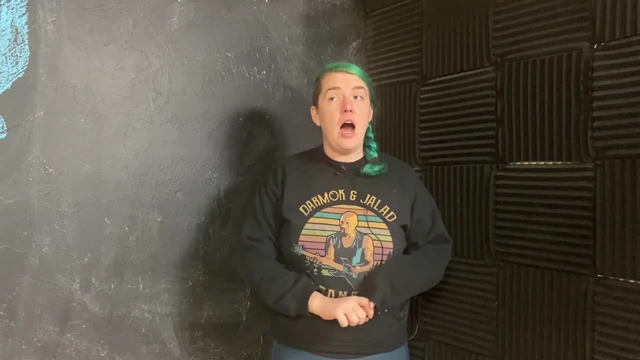 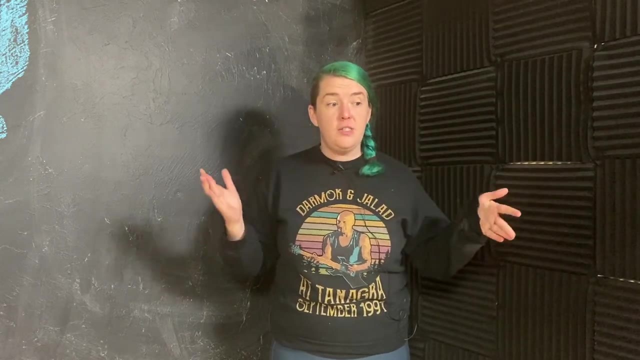 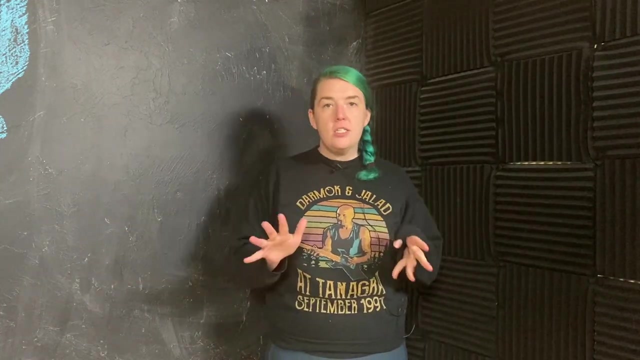 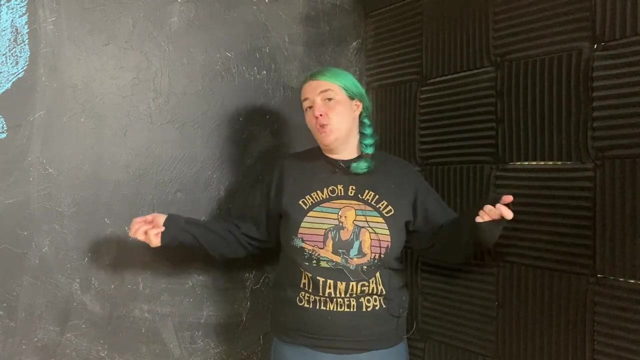 Other thing I currently filming. Maddie have no idea how long this video is going to be, So future editing Maddie, she's gonna know how long this is. She's gonna break this up into five-ish minute chunks, Because that's about as long as a normal. 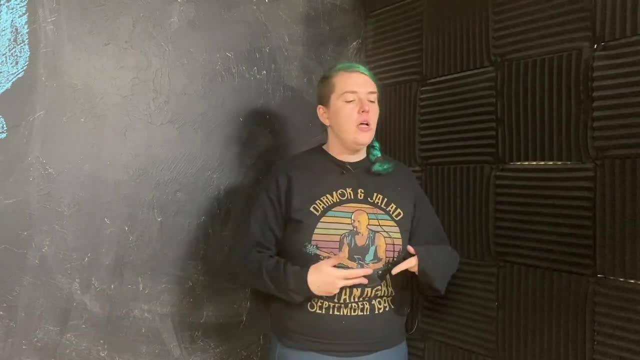 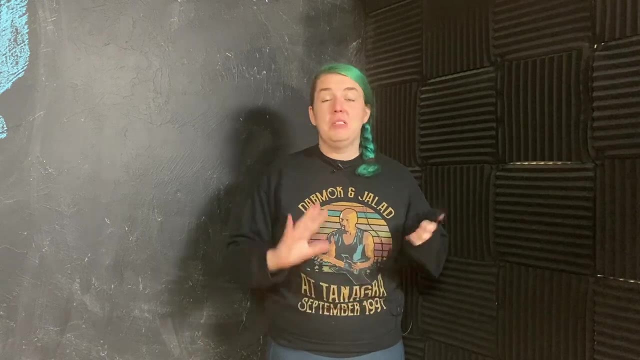 adult human's attention span turns out. So this video is going to have multiple parts, which are very important. It's going to be a lot easier to understand what's happening to parts, but at this moment I don't know how many. With all of that in mind, let's jump into this. 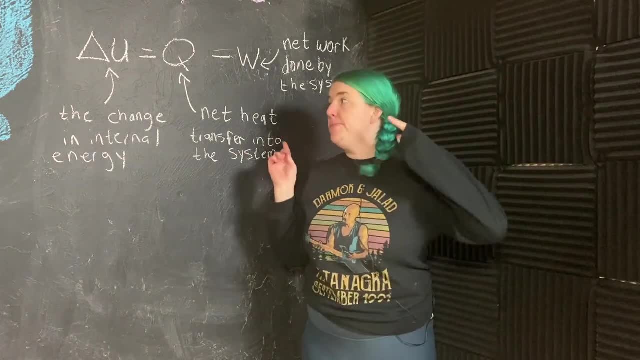 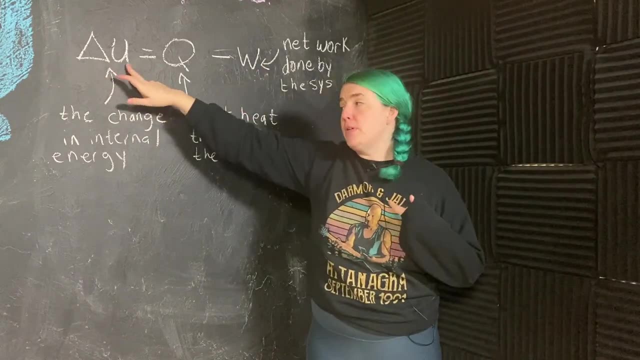 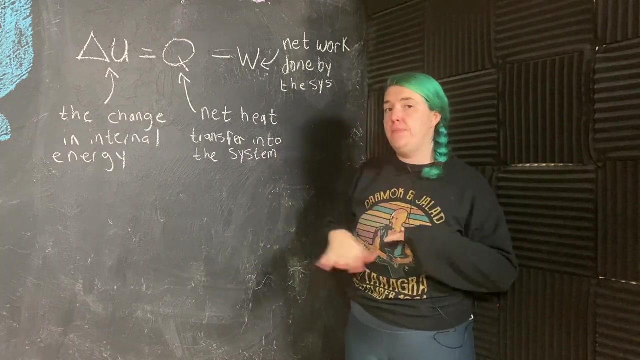 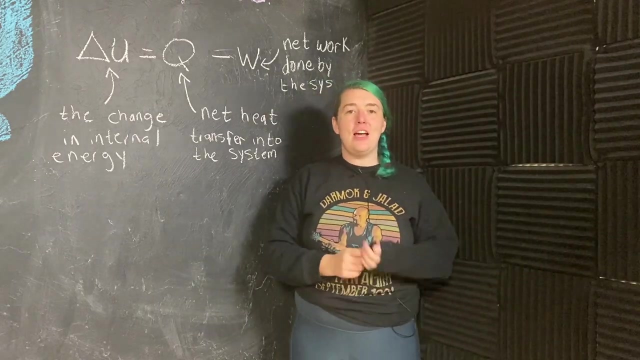 Mathematically, the first law of thermodynamics is this: Delta U equals Q minus W, where delta U represents the change in internal energy, Q is the net heat transfer into the system and W is the work done by the system. So anytime I see a new equation, the first thing that I want to think 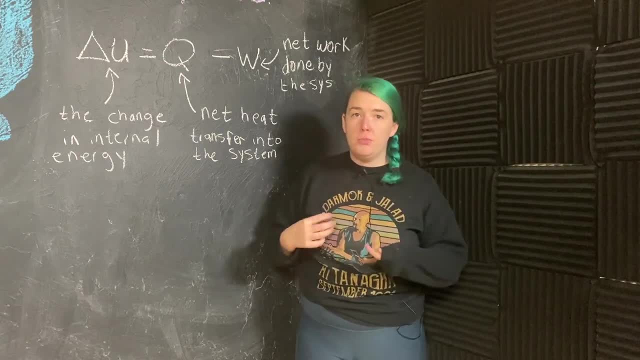 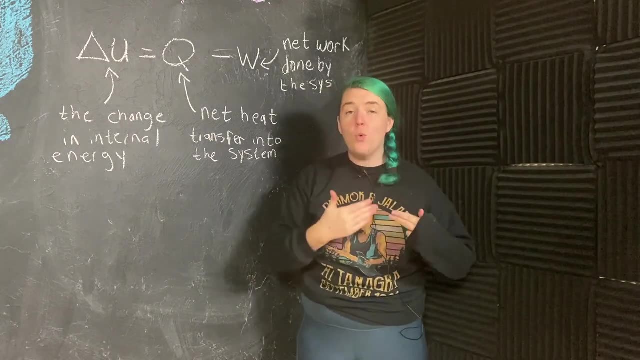 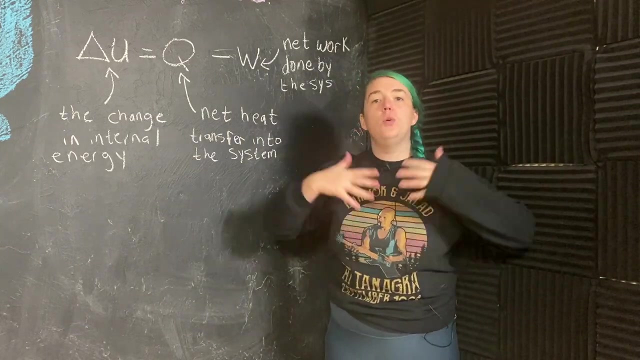 through is: what are the units of my terms? So all of these guys need to have the same units, otherwise we're trying to add apples to oranges and that doesn't work. So all of these guys have units of energy. energy That's going to be joules in the sort of standard SI system. Oh, you could think of it as 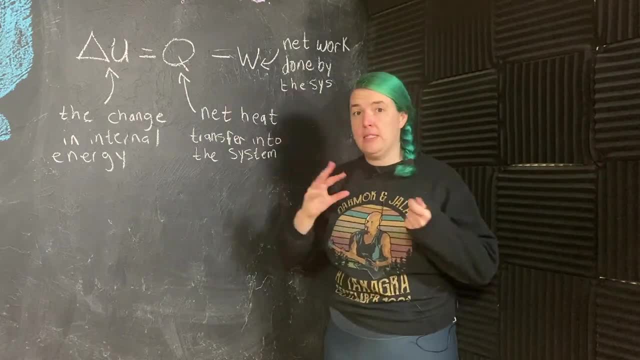 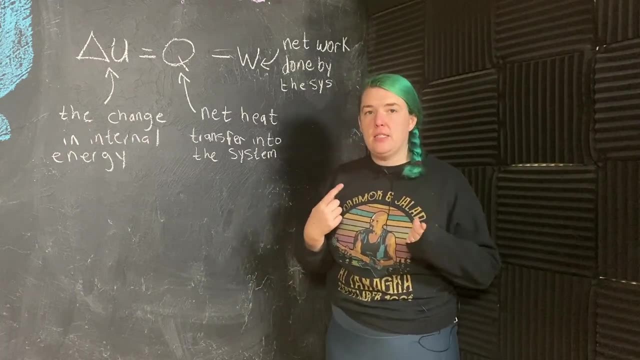 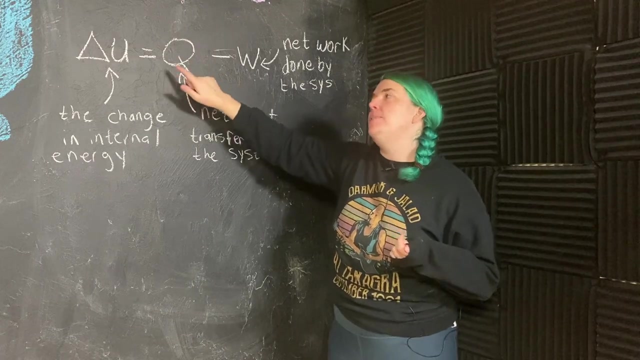 ergs. But fundamentally, all of these terms represent energy And since we know that energy can't be created or destroyed, what we're going to see is that if we say, add some heat to the system, we're going to add heat energy. Whatever I added here has to go somewhere. It can either. 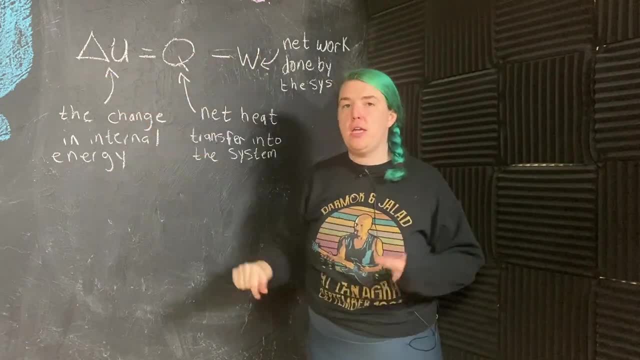 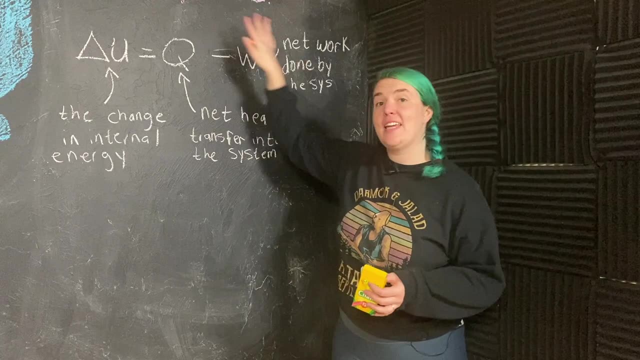 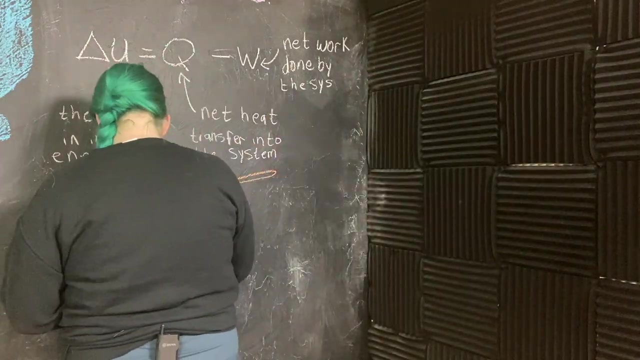 go to work, or it can go to internal energy, but we need it to be balanced somewhere. The system we're going to use to understand this equation is going to be a pot of water on the stove. Here's my pot of water, And the first thing we do is put our pot on the stove and then we're. 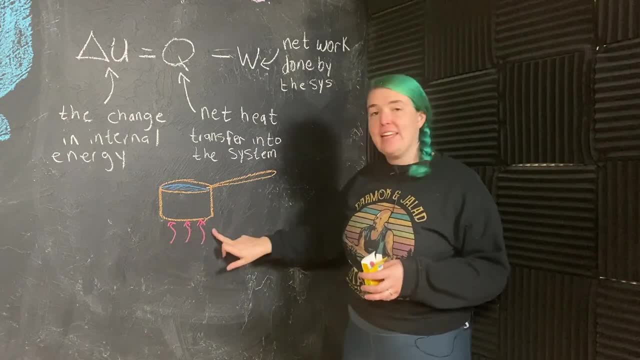 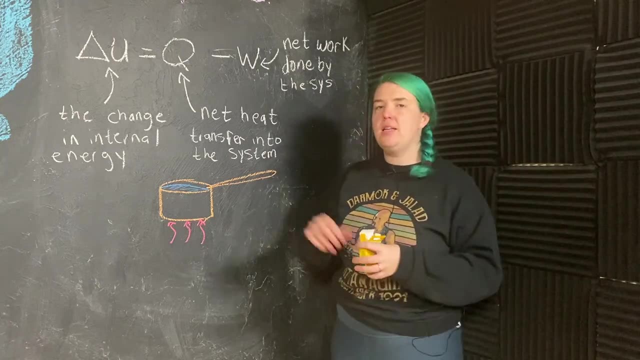 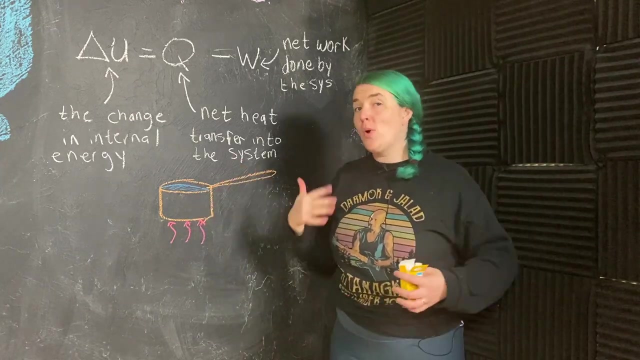 going to turn the burner on and start adding heat. So notice that we're now adding heat, creating energy. we're bringing in energy from the outside and dumping it into our system, where our system is the water in the pot. so we're adding heat, which means 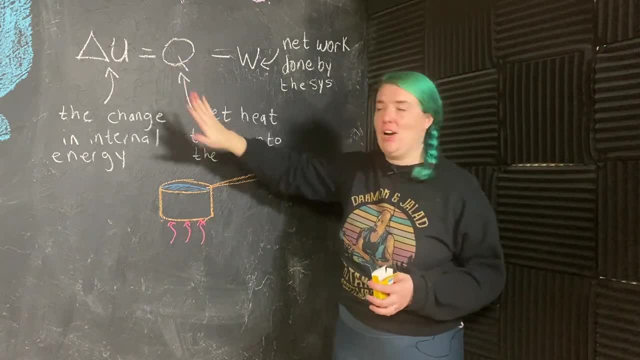 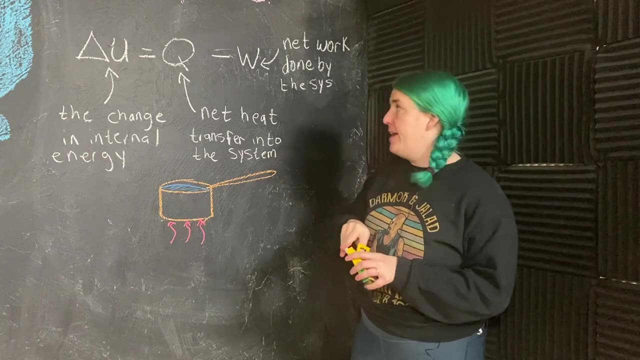 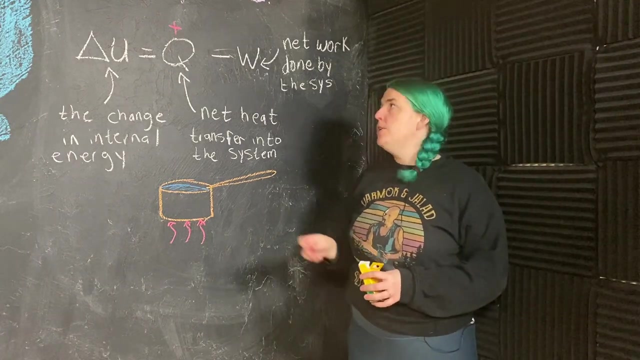 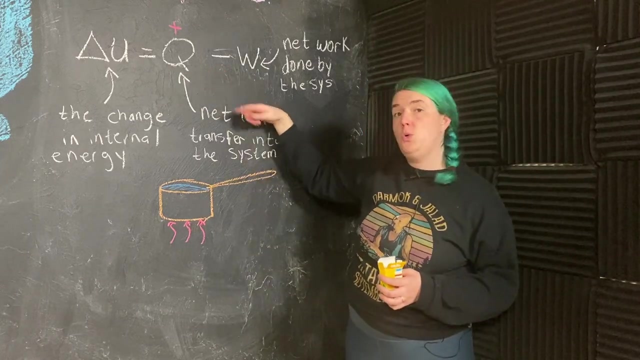 my Q value here is nonzero. we have some net heat transfer into the system, so let's go ahead and put a little positive sign there for our Q. so this heat, this energy that we're adding into this system, can only go to two places: it can go to doing work or it can go to the internal energy of the system. we could 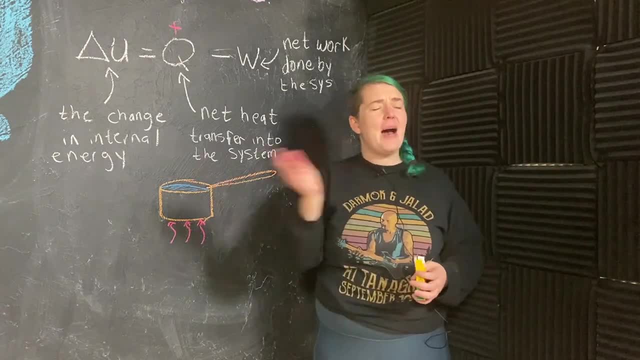 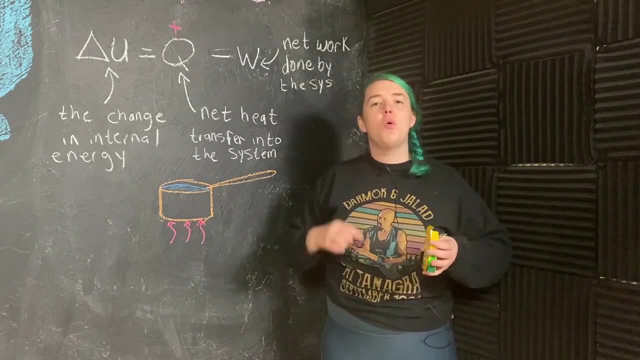 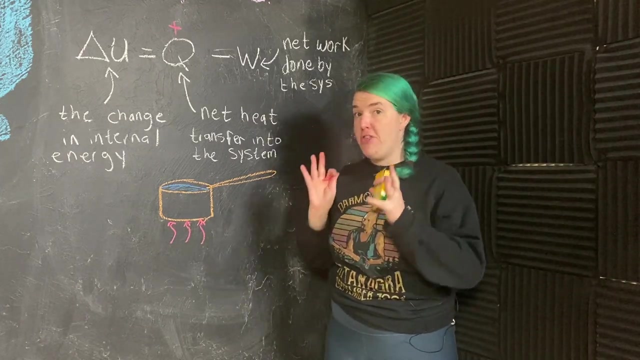 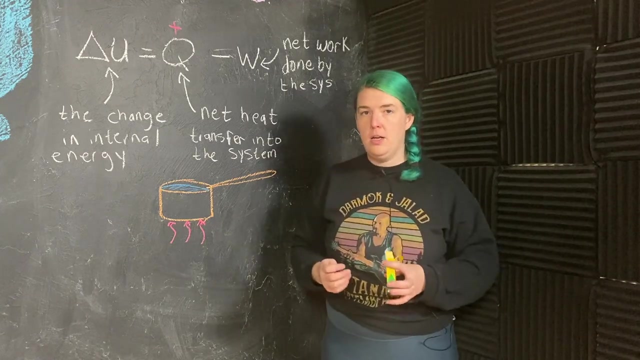 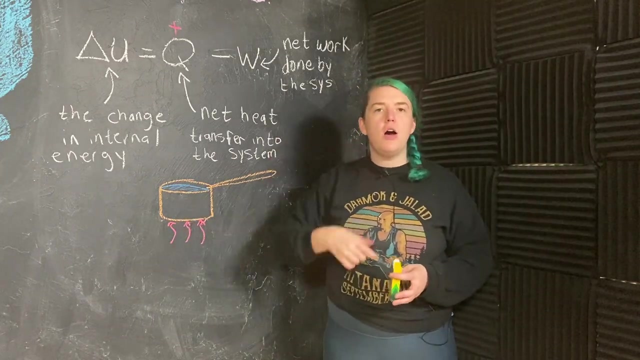 increase the internal energy of the system. now let's all think back to, like high school physics, where we learned that work is equal to force, times, displacement and arctic. so work is fundamentally related to physically moving things. if nothing is moving, then I am NOT doing work, and we're gonna see how. that very simple. 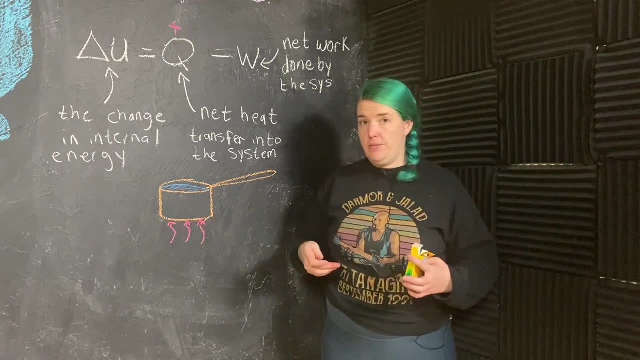 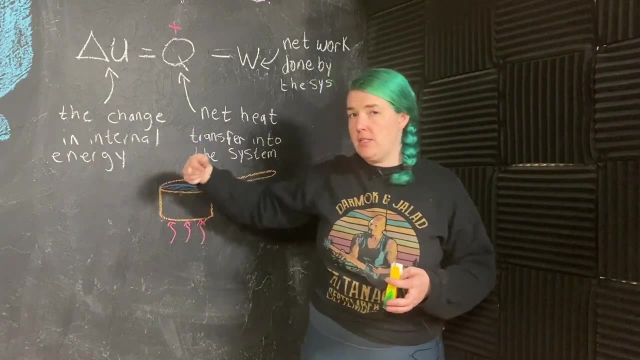 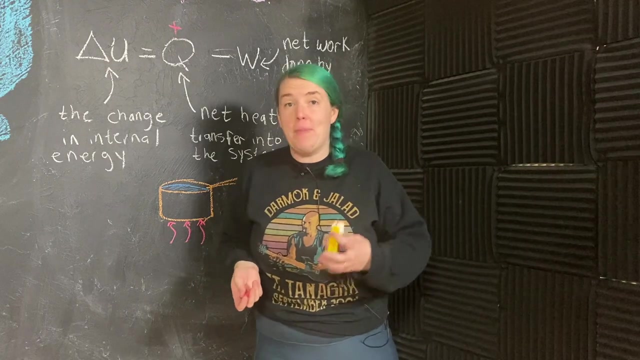 concept gets applied here. so when you first turn on that burner, the water is is changing the internal energy of the system. We're increasing the temperature of the water. Temperature is one of the ways we think about internal energy. It's not the whole story. 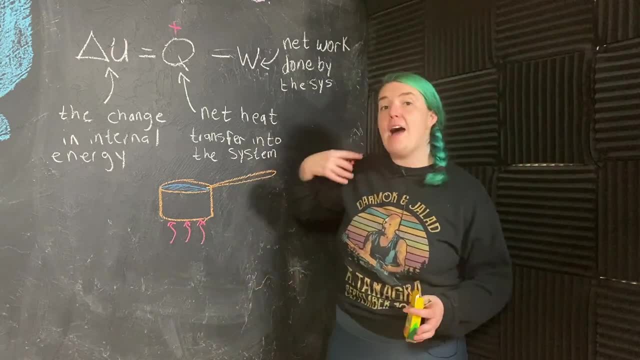 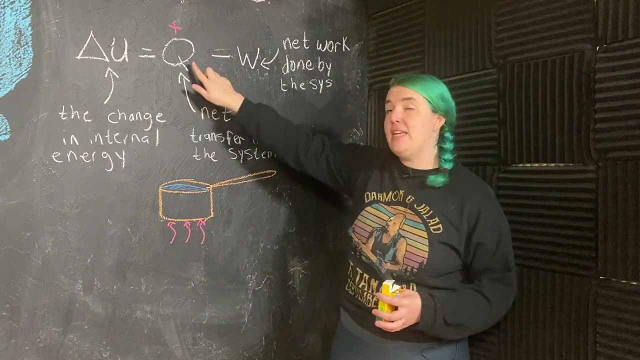 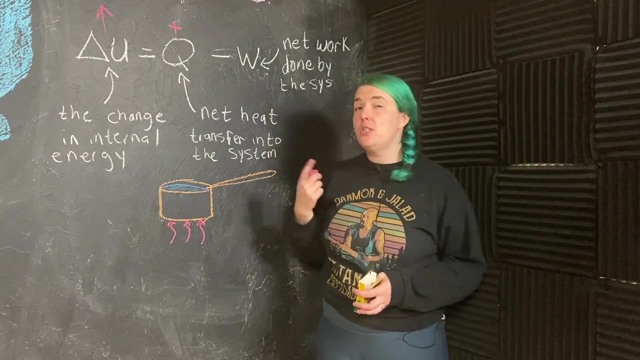 but it certainly is a big part of it. So at first, very specifically before the water begins to boil, all of my heat being transferred in goes to internal energy. The point at which this system starts doing work is when the water starts to boil.